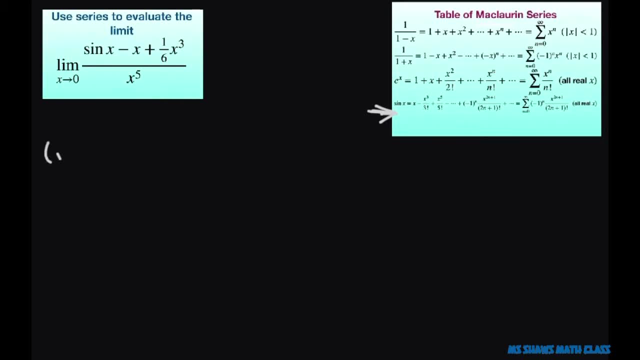 So I can just rewrite this as the limit as x approaches 0 and expanding sine of x. I'm going to get- I'm just looking at this- x minus 1 divided by 3 factorial times x. cubed plus 1 divided by 5 factorial times x to the 5th power minus 1.. 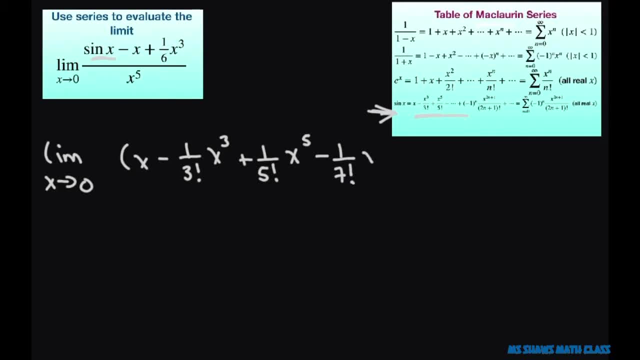 1 divided by 7 factorial times x to the 7th power, plus dot dot dot. And then we still have our minus x plus 1 divided by 6, x cubed, And our denominator is just x to the 5th power. 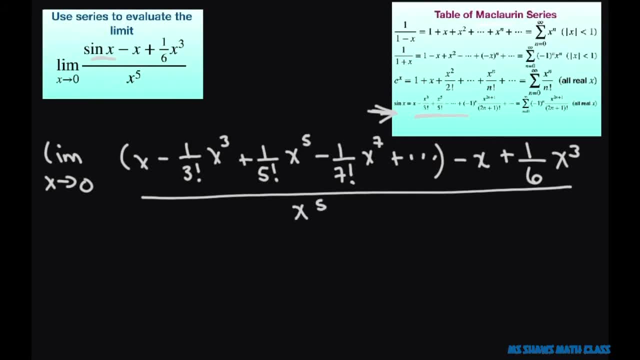 All right. Now what's going to happen is you get the limit as x approaches 0. These x's are going to cancel, And so are these two, because 3 factorial equals 6, which is 3 times 2 times 1.. 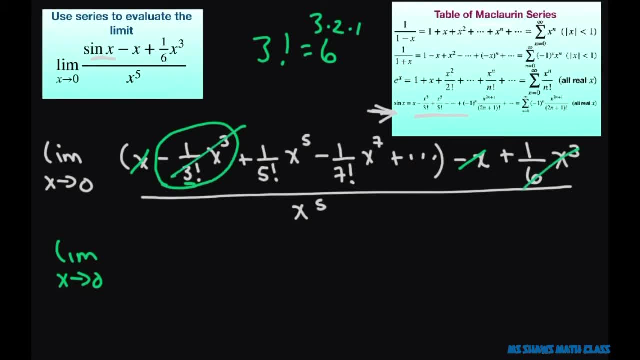 So these will cancel as well. So in the numerator you're left with 1 divided by 5 factorial times x to the 5th power, minus 1 divided by 7 factorial times x to the 7th power plus dot, dot, dot. 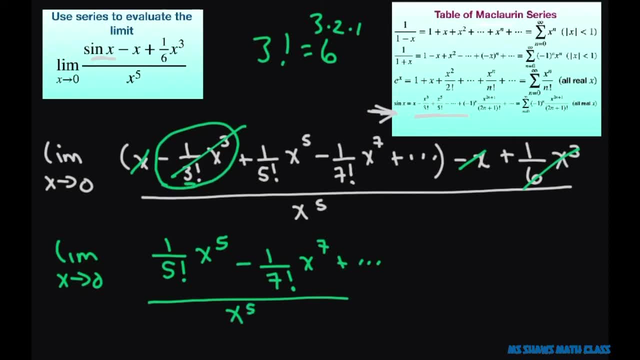 And then we're dividing by x: x to the power of 5.. So let's, since we're dealing with limits, let's just divide everything by x to the power of 5.. And if you do that, so I'm dividing each of these pieces. we're going to get the limit as x approaches infinity. 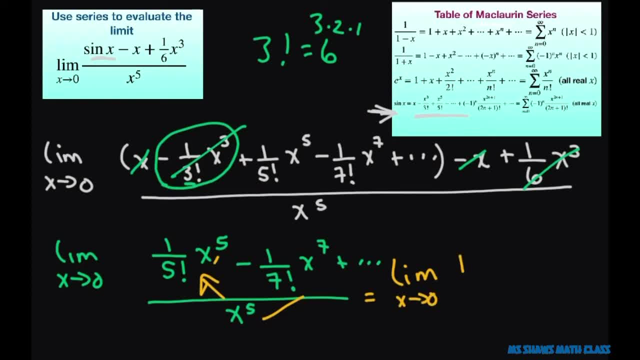 And these will cancel here. So you just get 1 divided by 5 factorial, minus x squared, divided by 5, 7 factorial. The next one would be plus x to the 4th, divided by 9 factorial, and so on. 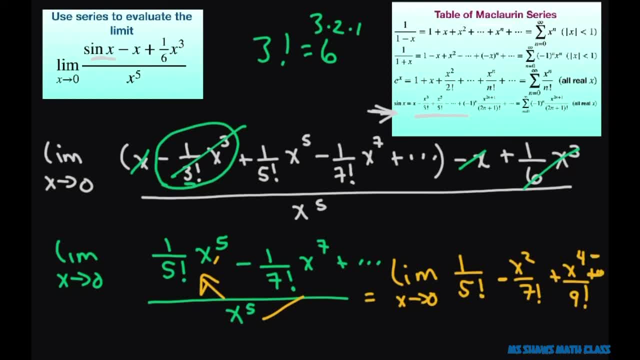 It would actually be minus, minus, dot, dot dot. Anyway, what's going to happen is all of this is going to equal 0.. So we're left with. this is your limit. So this equals 1 divided by 5..